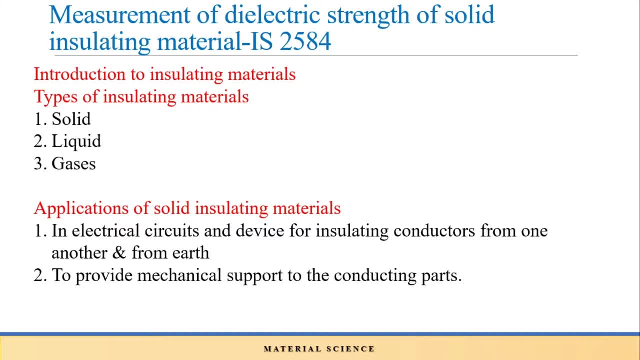 meaning of insulating material and dielectric material. so what is insulating material? so insulating materials are those which are not able to store a charge means they are used to provide a perfect insulation or they are provide us safety from the conducting material, whereas dielectric materials are those 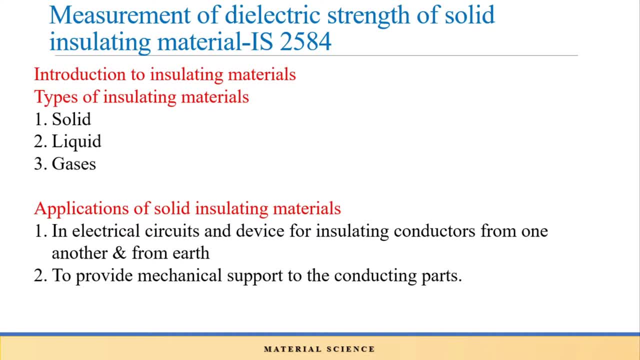 which are able to store some amount of charge in between them. we is from this. I can say: all dielectric materials are insulating material, but all insulating materials are not dielectrics. okay, so that is this basic difference between insulating and dielectric material. now we can classify the insulating material. 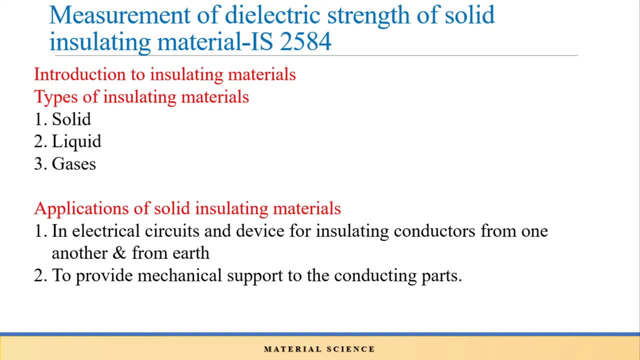 based on their physical state, as Dielectric material is insulated material based on its physical state as solid insulating material, liquid insulating material and gaseous insulating material. So here some in general applications are stated regarding the insulating material and at the last, 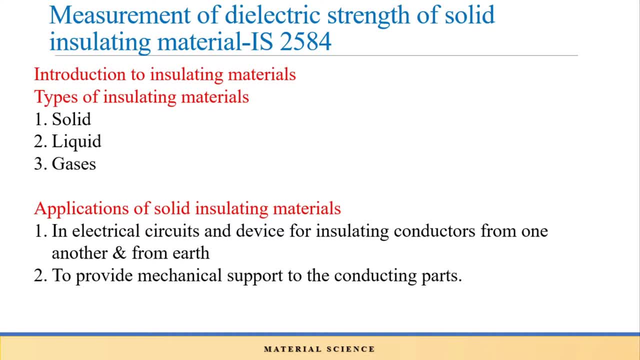 again. we will discuss in detail that. what which are the different applications of solid insulating material? So in general I can say insulating materials are used in electrical circuit and devices for insulating the conductors from each other or from the earth, as well as insulating. 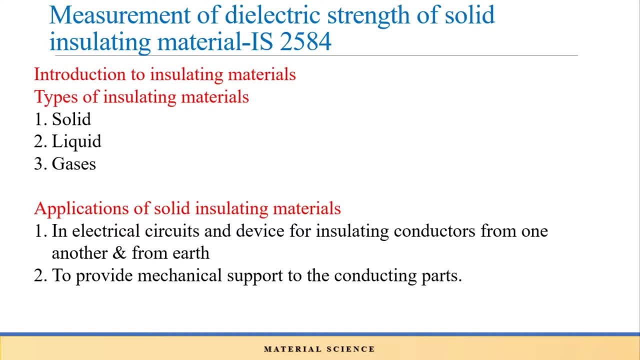 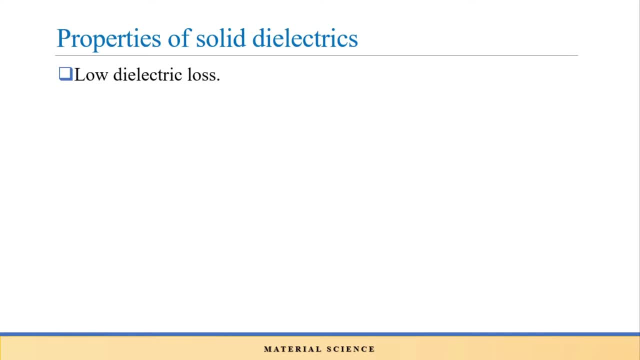 materials are used to provide the support to the conducting parts. So these are some general applications of solid insulating materials. Now, in short, we will discuss the different properties of solid insulating material. So first property is that low dielectric loss. So 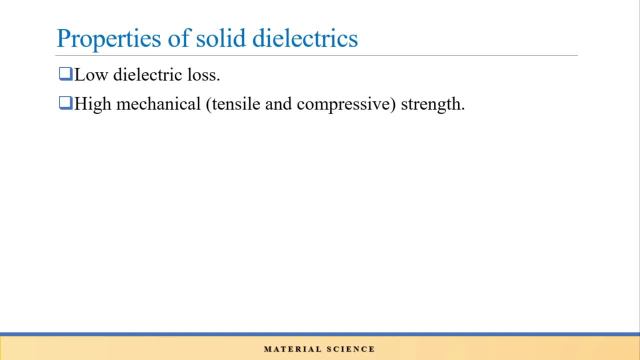 already. we are aware about the dielectric loss. So what is dielectric loss? So dielectric loss is nothing but conversion of electrical energy into heat energy inside a dielectric material. that is nothing but dielectric loss and that dielectric loss should be low in. 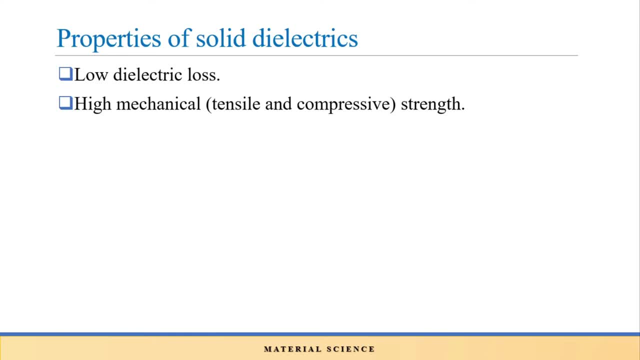 case of solid dielectrics or solid insulating material. Next property is high mechanical strength of this solid insulating material. So next it is: it should be free from gaseous inclusive or moisture. So obviously, if I am using some insulating material over the 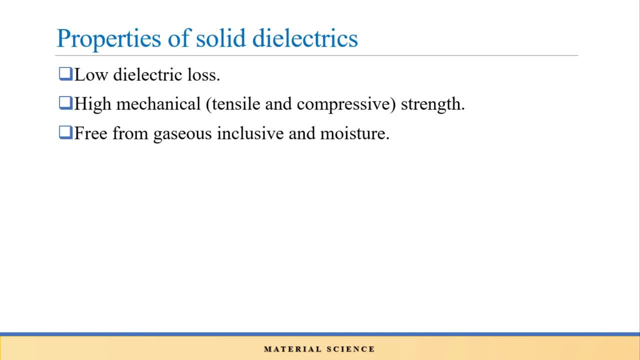 conductors, then it should be free from gaseous inclusive or moisture. So obviously if I am conducting part, then it should be free from moisture's content as well as it should be free from some gaseous inclusives. So if there is presence of some moisture's content, then that. 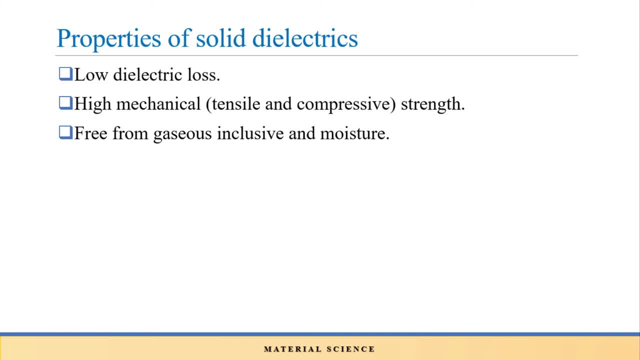 solid insulating material is not able to provide a proper insulation. that's why it should be free from the moisture. Next, resistance to thermal and chemical deterioration. Obviously, if I am using some insulating material, then it should be resistive to the thermal and chemical. 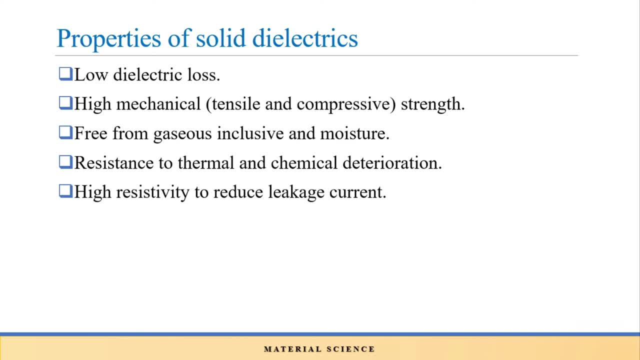 deterioration properties. Next, property that is high resistivity to reduce leakage current. So if I am having some insulating material which is provided, or the conducting part, then there is some amount of leakage current which is radially flowing outward in direction and the function. 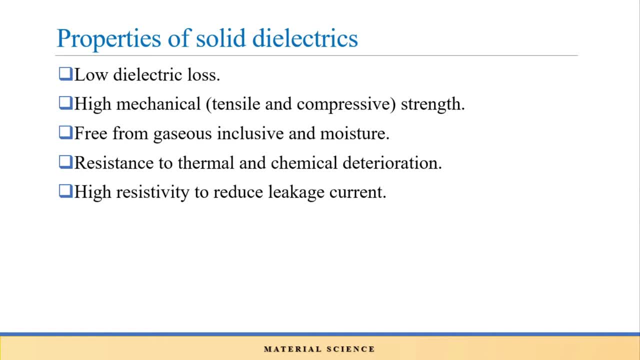 of the insulating material is to suppress that leakage current. So obviously a ideal solid insulating material will suppress or will reduce thevisual range of water vapor to theornoil at the leakage current from that conducting part. Next they should have high dielectric. 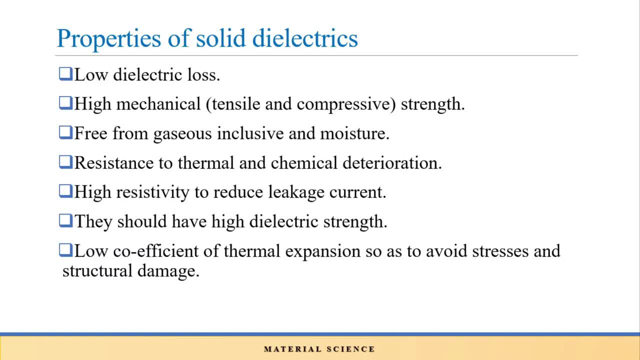 strain. so obviously, if an insulating material is having high dielectric strain, then it will be used like a good insulating material After that low coefficient of thermal expansion, so as to avoid stresses and structural damage. So practically, it may happen that due to certain physical conditions, a 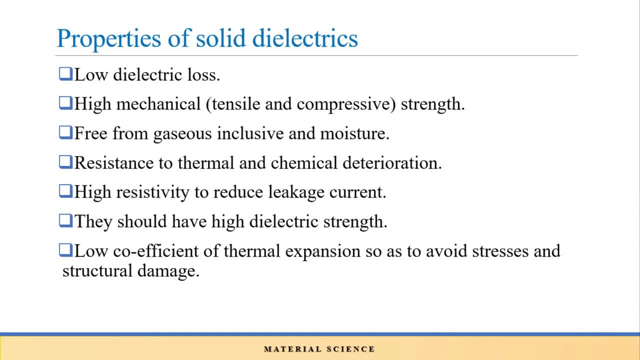 temperature at a particular point may exceed some beyond range and in that case that insulating material may start expanding and which will reduce the insulation properties of that insulating material. So practically there should be low coefficient of thermal expansion of a good insulating material. Next again I 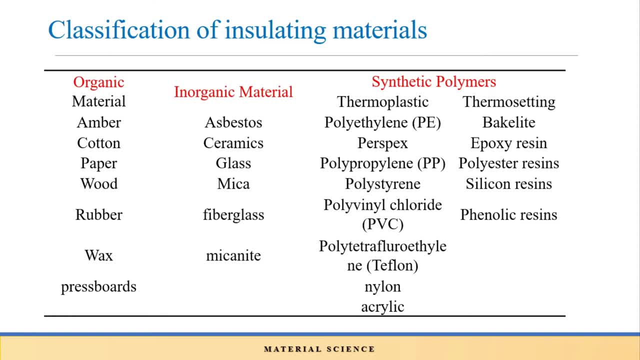 can classify the insulating material as organic material, inorganic material and synthetic polymers. So some examples are stated here. that is amber, cotton, paper, wood, rubber, wax, press board. these are the examples of an organic materials. So organic materials are those. 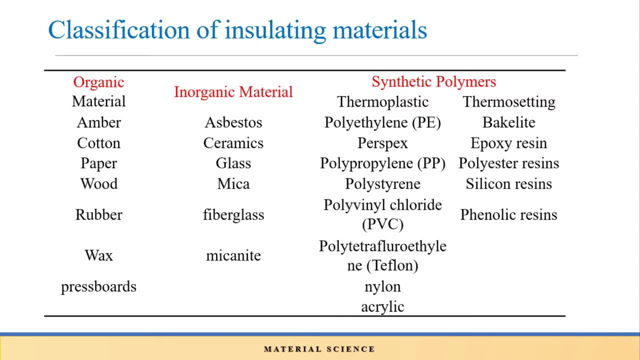 which are naturally available or they are taken from the trees or plant, So inorganic materials. so some examples of inorganic materials are asbestos, ceramics, glass and some synthetic which are obtained from some polymerization process. Again, in case of synthetic material, there are two types. one is 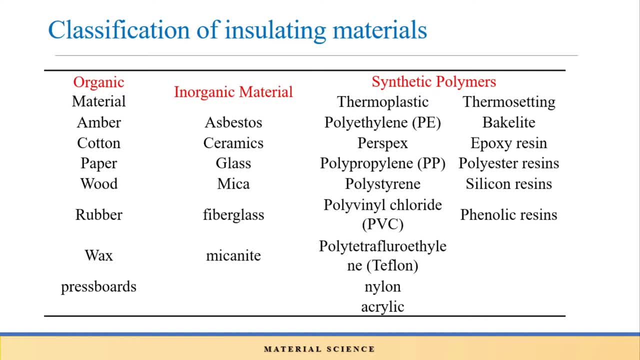 thermoplastic and another one is thermosetting. So we will have in some detail the thermoplastic and thermosetting polymers and some examples are stated here, as a polyethylene as a synthetic polymer and bacallite as a synthetic polymer. So in detail you can read all these examples and in upcoming 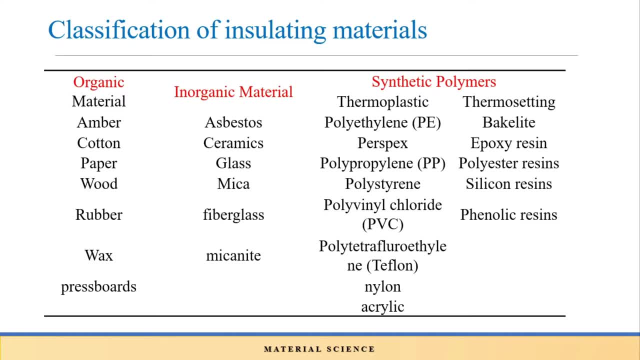 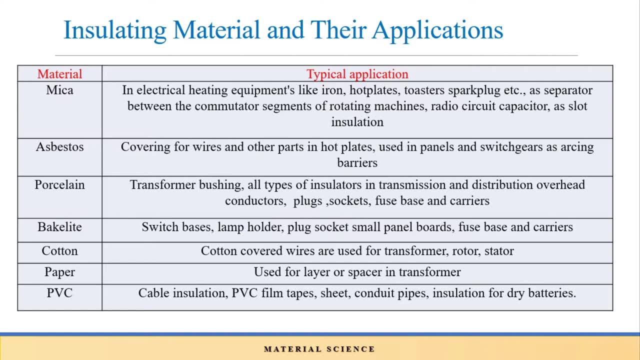 unit. we will have detailed study on these classifications of the materials. So, again, if I am considering some solid insulating material, and here some applications are explained of that solid insulating materials, So you can go this table that is mica, asbestos, porcelain, bakelite, cotton paper and PVC. So in detail, 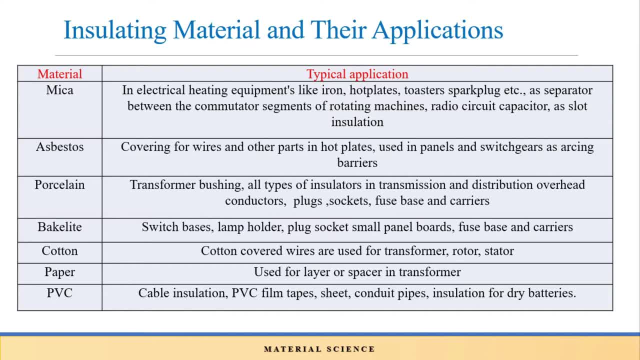 here I have explained where I can use the mica as well as where we can use the asbestos. So again, this part may be discussed in later on or in the next unit. but here we need to focus on the testing of solid insulating material So we can choose any material for the testing from. 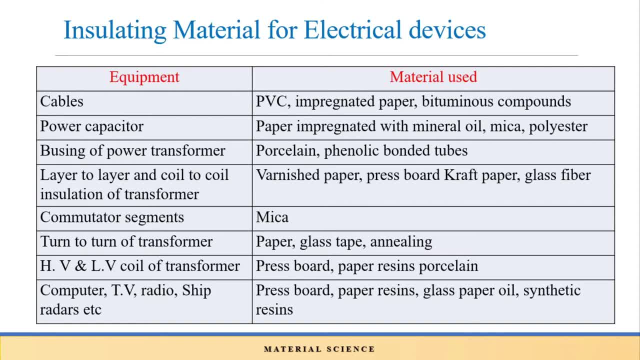 these given materials. Next, insulating material for an electrical device. So in which equipment which type of material is used? in this table means if I am having cable then I can separate the different insulating materials used in cable that maybe PVC impregnated. 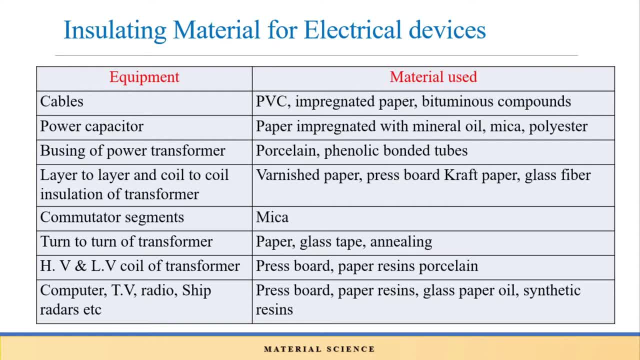 paper. Likewise, I can separate the material or insulating material which are used in cable. Again, if I am cutting账, considering the power capacitor, then again I can separate the materials used inside a power capacitor. that may be paper, mineral oil, mica, polyester. Likewise, in this table explained each 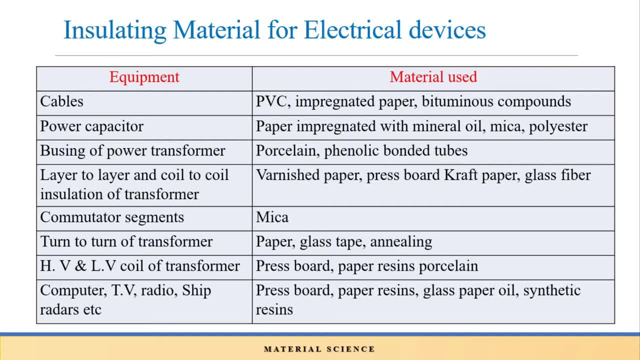 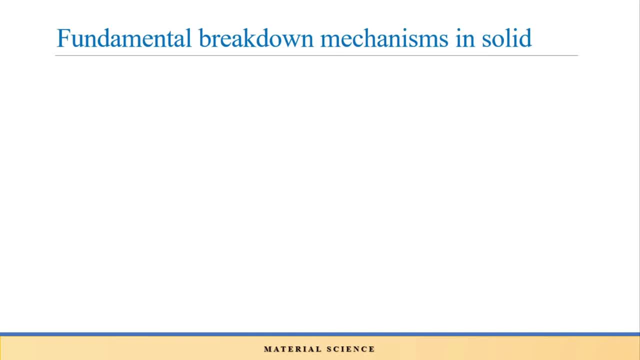 equipment and different materials used under that electrical equipment. So you can go through this. So let us discuss the next point. that is fundamental. breakdown mechanism in case of solid insulating materials means how the breakdown will takes place in case of solid insulating material. So first point is intrinsic breakdown, So some electrons are able to move through the 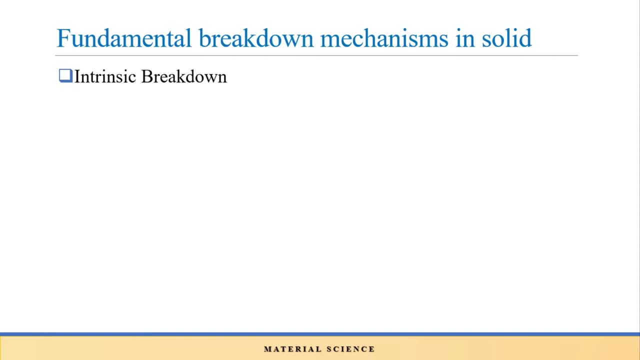 lattice factor of that solid insulating material and that type of breakdown is known as a intrinsic breakdown. Second one is thermal breakdown. So we know that some dielectric loss is taking place inside a insulating material. means some electrical energy is being converted into heat energy and 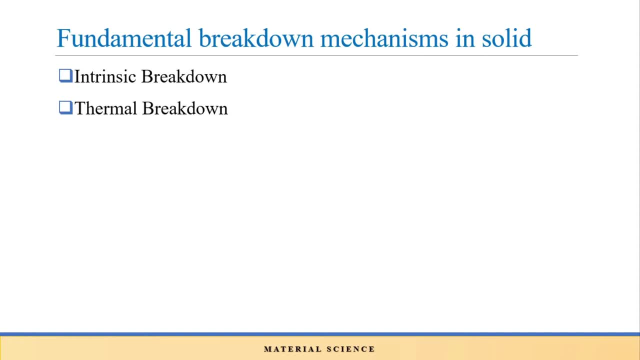 due to that generated heat, the insulating material may get expand up to certain level and from that point some electrons are able, or some leakage current is able, to flow through that insulating material and such type of breakdown is nothing but thermal breakdown. Next breakdown due to internal discharge. So we know that at the time of 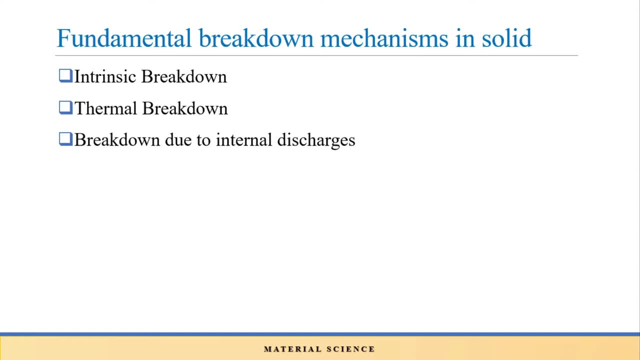 manufacturing process. some voids or gaps means it is a manufacturing fault which is present over that insulating material. and as you are applying an electrical pressure to such insulating material, then up to certain or over the certain limit the electrical pressure may get created on the surface of that insulating material and if some gaps or voids is present, then leakage current. 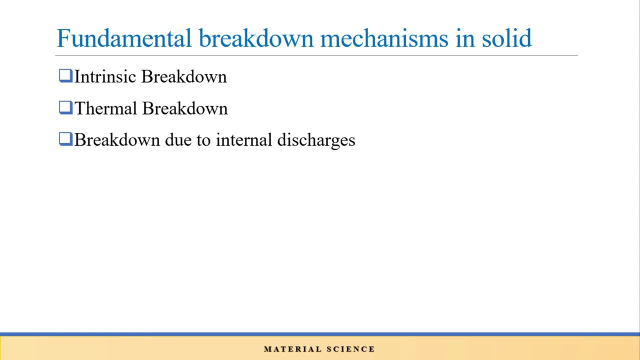 will flow through that gap or voids, and such type of breakdown is nothing but internal discharge type of breakdown. Next breakdown is of electromechanical type breakdown. So electromechanical means what? when we are applying an electric field to an insulating material, then there is a formation of polarization. 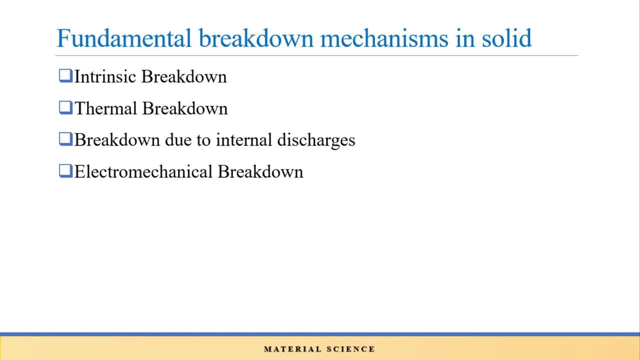 and when polarization will occur, then there is a deposition of two oppositely charged particles on the electrode and they are responsible for the breakdown. and such type of breakdown is known as electromechanical breakdown, Next electrochemical breakdown. So if there is a presence of some chemicals or an insulating, 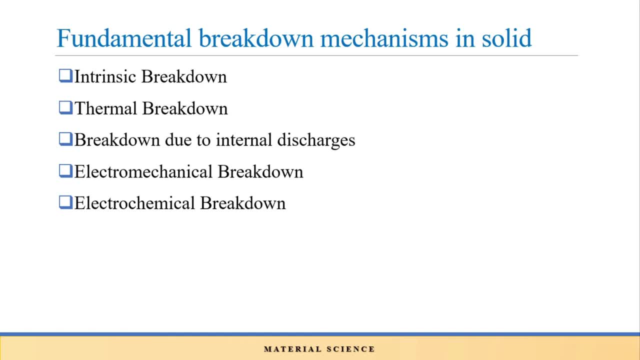 material, then which then it is responsible for the transfer of electrons, and such type of breakdown is known as a electrochemical breakdown, Next breakdown due to surface discharge. So we know that on the surface of insulating material, if there is a presence of some 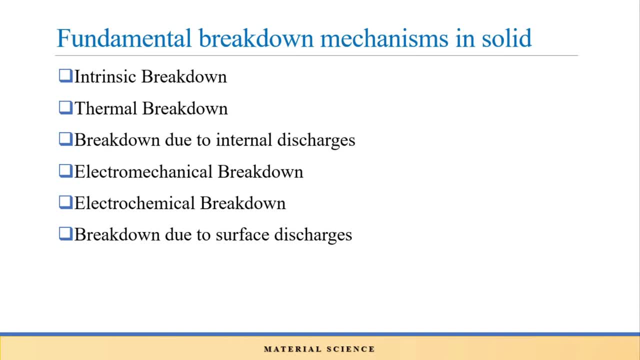 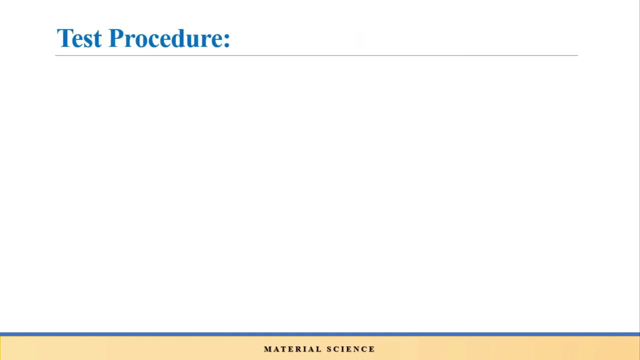 moisture or dust content, then they will allow us to some extent to pass the electric field through that moisture and they are helping us to breakdown of an insulating material. So such type of breakdown is known as a breakdown due to surface discharge. These are the some fundamentals by which breakdown will takes place in case of solid insulating. 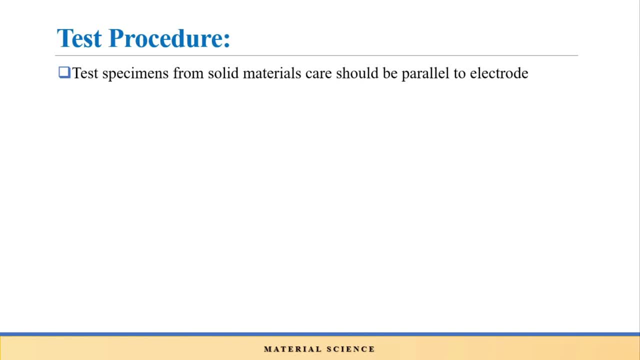 material, How to measure the breakdown strength of a solid insulating material. for that we are having a procedure. so here we will discuss one step by step the test procedure to conduct the breakdown test on solid insulating material. So first step: test specimen from solid material. care should be parallel to the electrode means. if I am taking 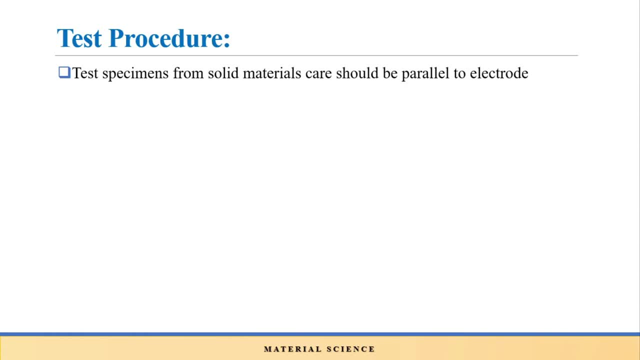 one piece of paper and I am trying to find out the breakdown strength of that paper, then that paper should be kept parallel to in between the two electrodes. Next, the area of the test specimen should be sufficient to prevent flash over means. the size of that paper should. 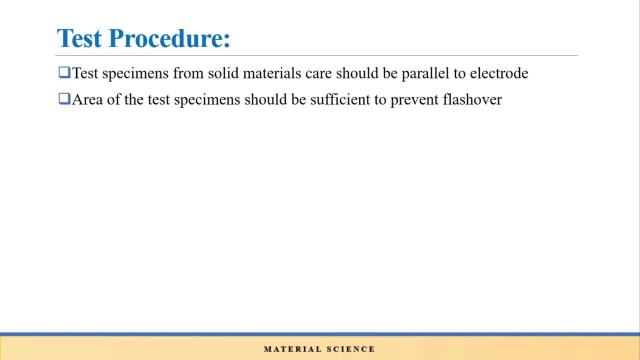 should be enough, which will cover the surface of the electrodes. Next, the electrode should be kept clean and free from pitting caused by an arching. So every time when I am testing the different materials, then at that time you should clean the surface of electrodes. Next, there should 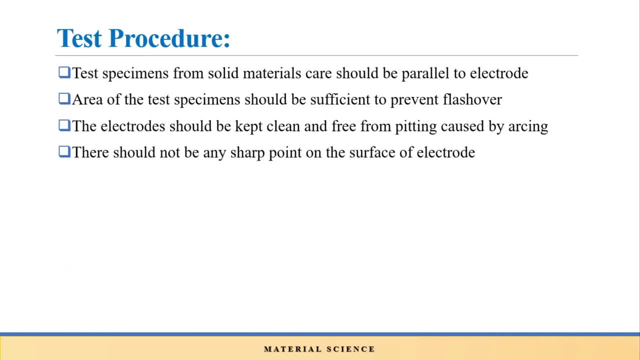 not be any sharp point on the surface of electrode. So obviously, take care that the electrodes which are used for the testing purpose they are smooth in nature. there should not be any pointed surface lying for the surface of electrode, which will cause an early breakdown of an solid insulating material. Next, ensure that the test cell is properly connected. 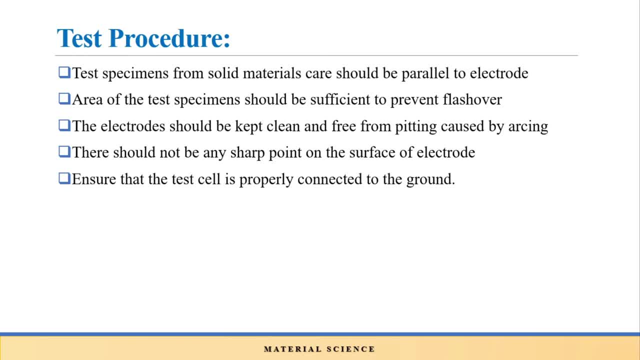 to the ground. so obviously, if we are working on a high voltage, then the test cell should be connected to the ground. Next, place a sheet of insulating material in between the two electrode properly. so obviously, as we have discussed in the first point, the test sample should be placed. 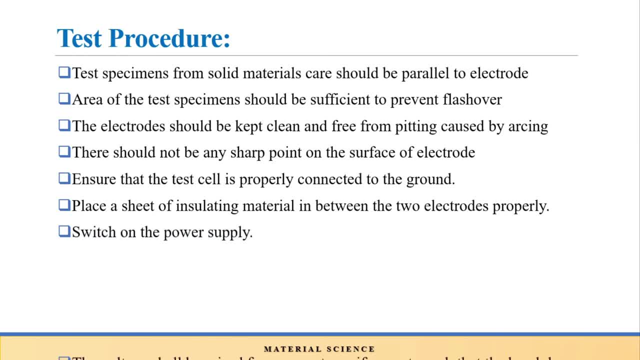 properly in between the two electrodes. Next switch on the power supply and after that next the voltage shall be raised from zero at a uniform rate, such that breakdown will occur. So take care that you are varying the voltage by uniform rate. it may be 2 kV per second. Next note down the exact 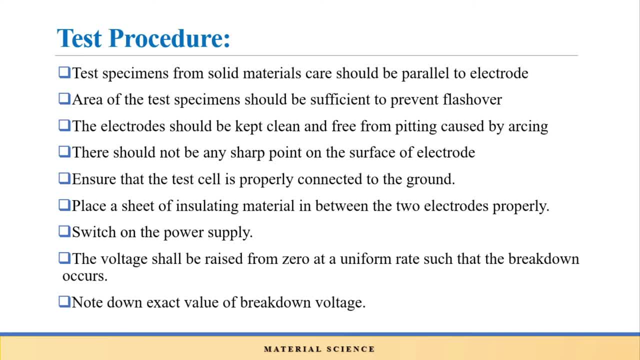 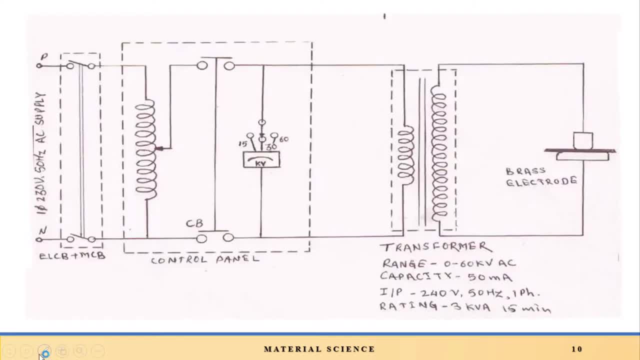 values of breakdown voltage, and after the test sample should be placed properly in between the two electrodes. Next switch on the power supply and after reading the breakdown voltage you can find out the breakdown strength of solid insulating materials. So here some basic diagram is explained here. so first of all, here I am having phase and 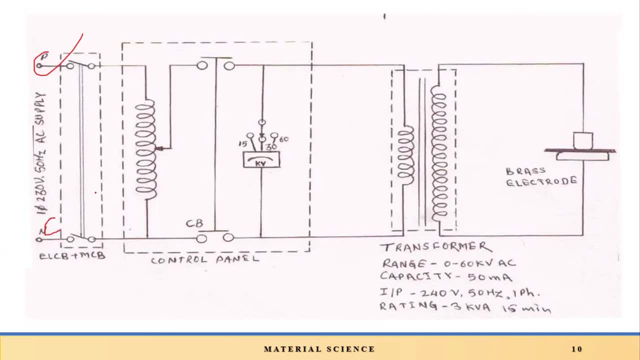 neutral, and after that you can have ELCB and MCB arrangement, and then I am having atotransformer. in order to vary the voltage, here step up transformer is used. this is the primary side and this is a secondary side In which higher voltage will be present. and here test sample is present means two electrodes and 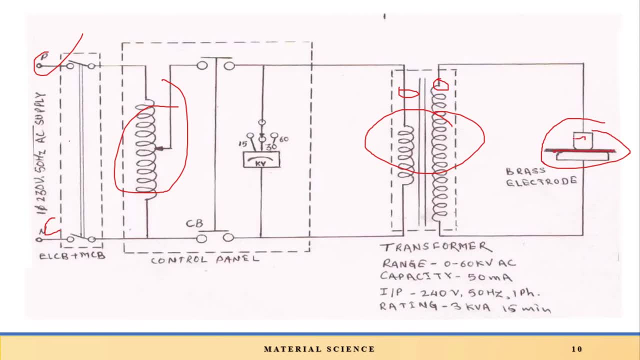 in between that. this is the test sample, so this is the upper electrode and this is the lower electrode, and in between that, one test sample that may be paper or anything which is placed in between these two electrodes. okay, so here you can write down the rating of the transformer used. 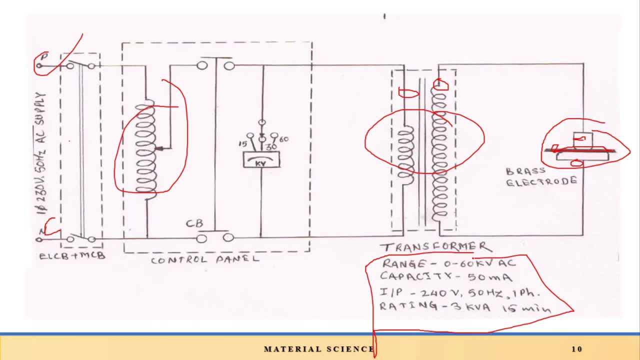 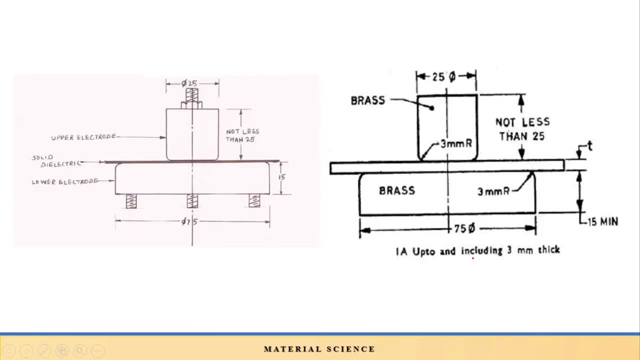 that which is nothing but zero to sixty kV, or and that is depend on the temperature of the transformer. So this is the laboratory setup. okay, so every lab will have different specifications. so here one simple diagram which will show us the nature of the test cell. means this total is a lower electrode. 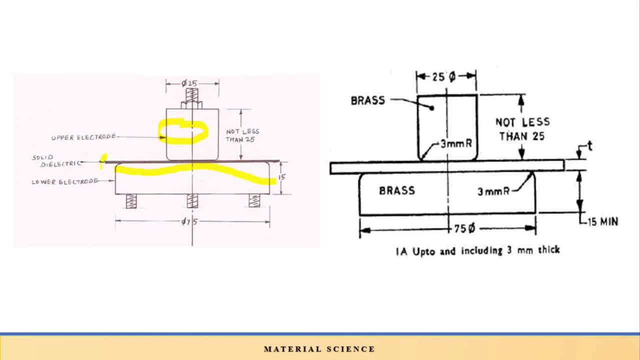 this one is a upper electrode and in between that I can place a test sample, so solid insulating material that may be paper or piece of paper, which is placed in between these two electrodes and I can apply the test sample. So this is the variable voltage and at a particular point this material may get break and one can measure. 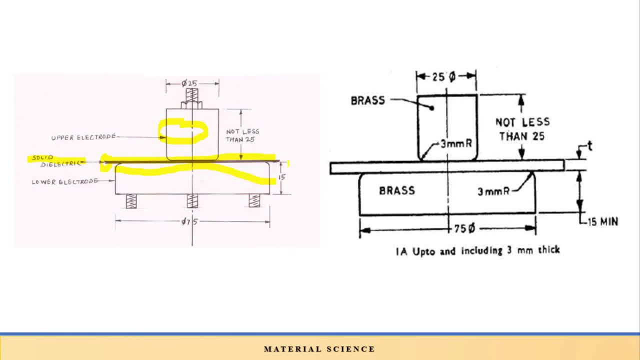 the breakdown strength of that solid insulating material. so here some specifications are explained according to IS standard. that is, height, length or what is this? length of the upper electrodes and diameter, everything which is given in the IS standard. okay, so this is the standard diagram from book and it which is can be drawn on the notebook. 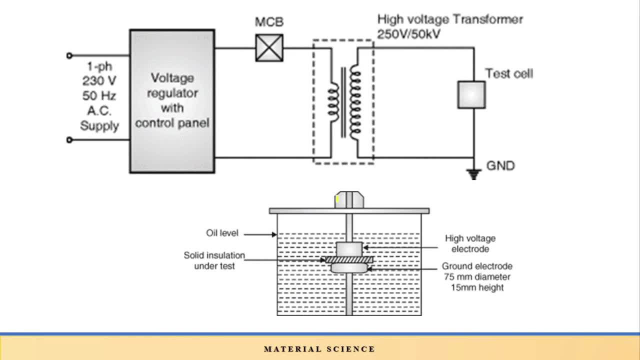 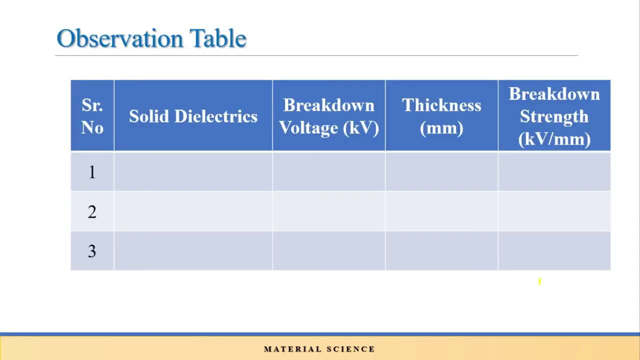 Next. so this is the ideal circuit diagram. so in previously we have drawn the diagram with the help of pen and this is from the textbook, and here they have mentioned the ideal test cell. Next, observation table. so after testing the solid insulating material, we have to mention: 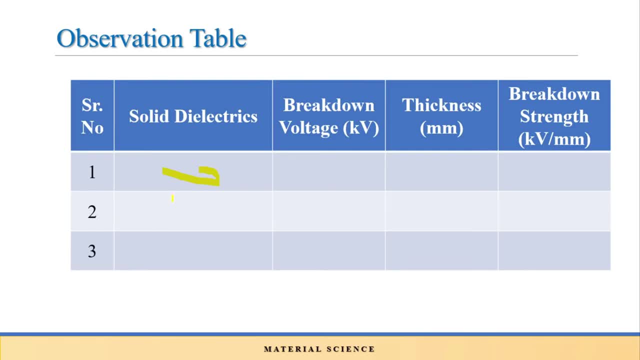 here which type of solid insulating material used means that may be paper or asbestos or mica sheet. You can explain. Name that material here. after that, what is the breakdown voltage? that may be 4kV, 5kV or 6kV, anything, so that last breakdown voltage recorded can be written here and then finally, 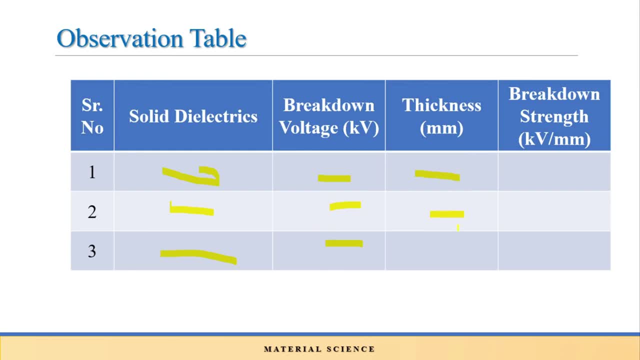 thickness. so we have to measure the thickness of that test sample and that can be noted down here. so I can mention that may be 2mm, 1mm, 0.5mm, likewise, so that is depending on the material or which material is used for the testing purpose. and finally, I can have 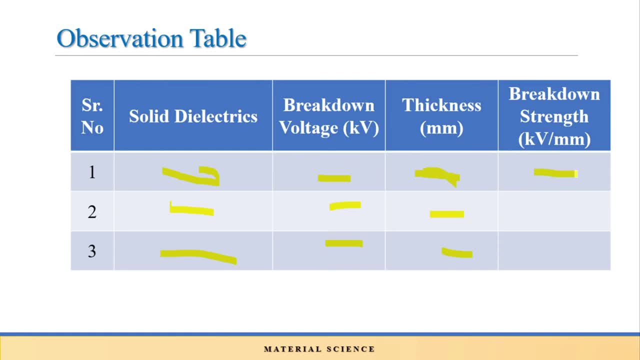 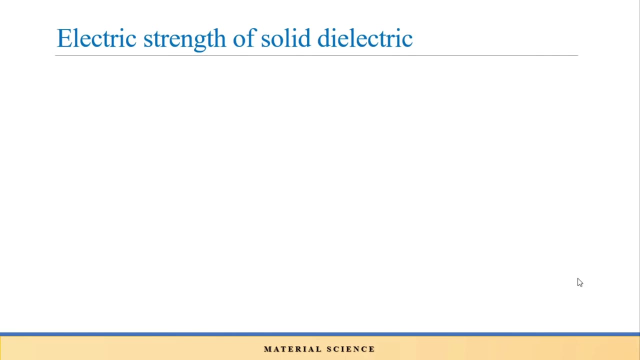 I can calculate the breakdown strength of the material by kV per mm means. this is the breakdown voltage divided by thickness of that material, which is nothing but breakdown strength of the material. and here you can mention that breakdown strength for each and every material as kV. 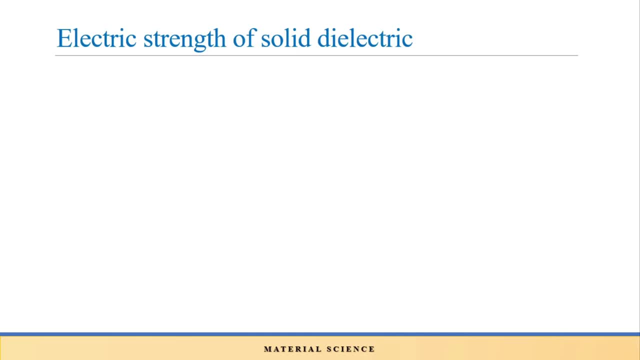 Next, the different factors which are affecting on the dielectric strength of solid insulating material. so first, thickness of the material. so as there is increase in thickness breakdown voltage is increasing, but breakdown strength may remains same temperature. so if there is increase in temperature again, breakdown voltage may get reduced. moisture content. so 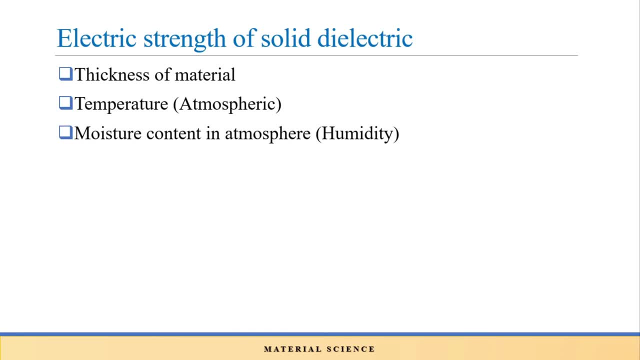 if there is presence of any moisture content on the surface of solid insulating material, then again it will affect on the breakdown voltage. again duration of applied voltage that will affect on the breakdown voltage of solid insulating material. Then composition of the material. So this is the breakdown voltage. 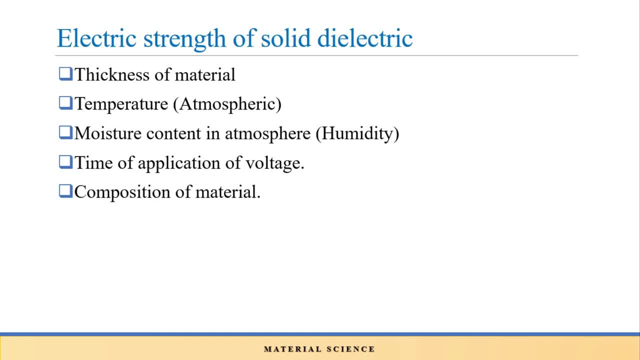 The composition of the material means whether the composition is organic, inorganic or synthetic. based on that, its breakdown voltage is different for the different type of solid insulating material and defects of the material. so if there is any white or gap is present on the surface of that material, which will again affect the breakdown voltage of solid insulating.